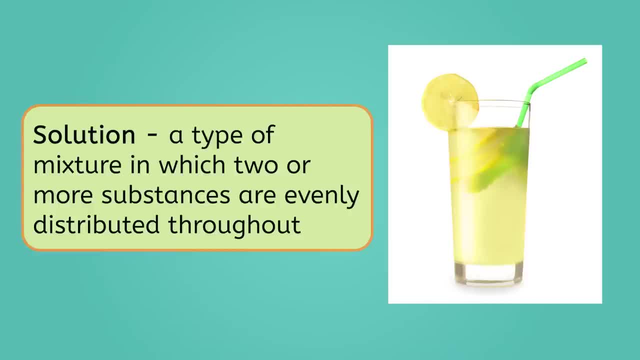 which the substances are evenly distributed or spread throughout it. We can't see the substances that are in the same state of matter. We can't just reach in and pull out just lemon juice or just sugar the way we can with some other mixtures. Some other examples of solutions. 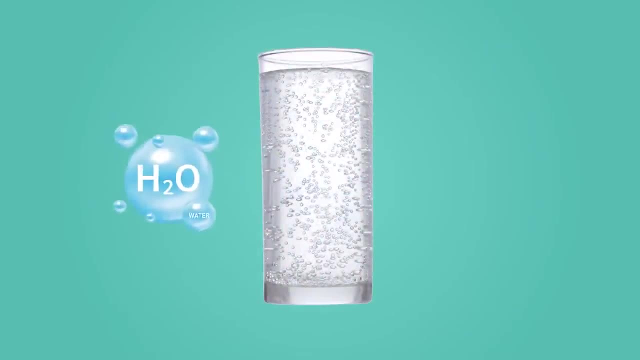 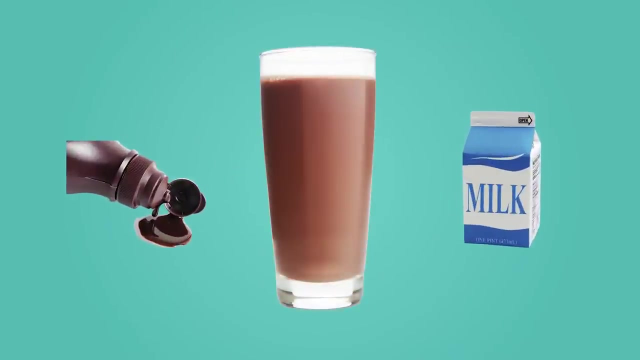 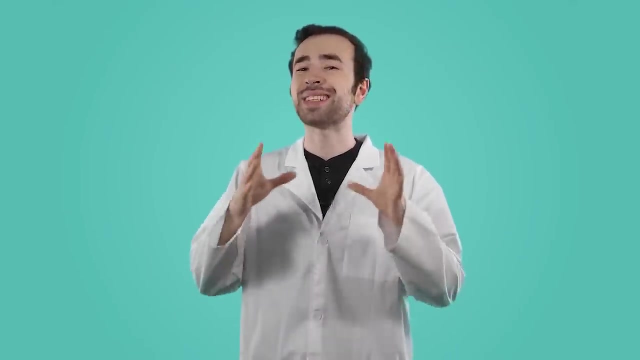 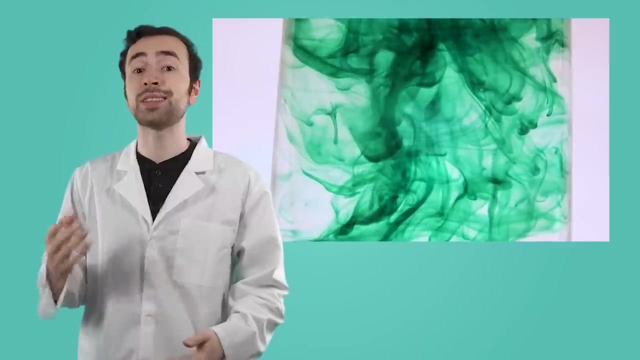 include sparkling water, which is a mixture of water and carbon dioxide, or chocolate milk, which is a mixture of well, chocolate and milk. Solutions are often made using different substances that are in the same state of matter, like food coloring and water, But you can also make a solution out of a solid and a liquid. Remember in a previous lesson. 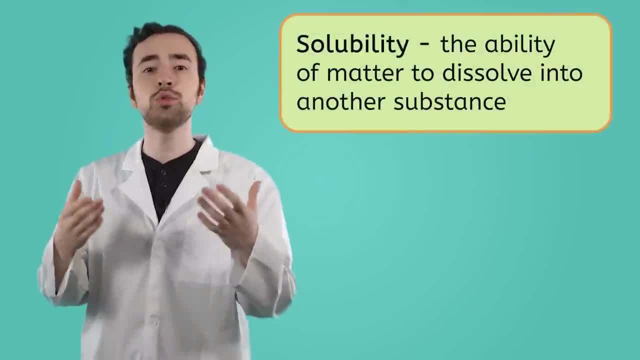 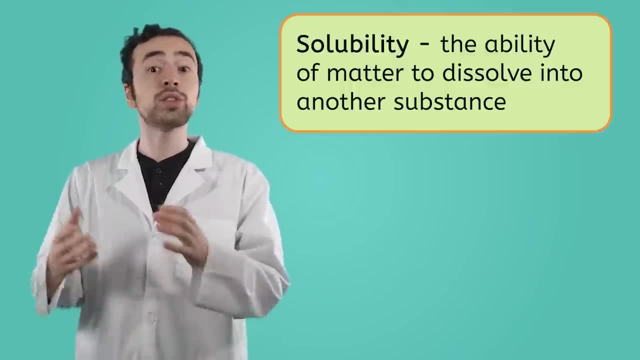 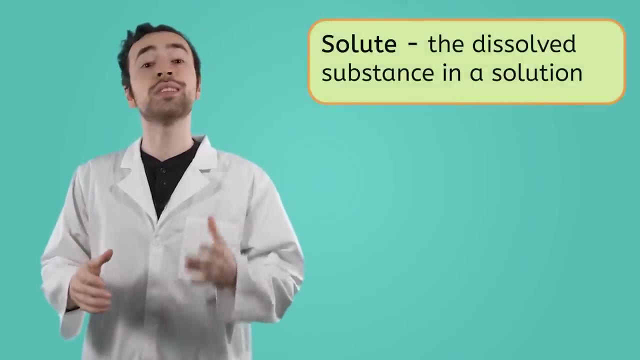 about the physical properties of matter. we learned about solubility, which is the ability for matter to dissolve into other substances. Well, when a solid dissolves into a liquid, you get a solution. The solid that is dissolving is called the solute and the liquid that the solid is. 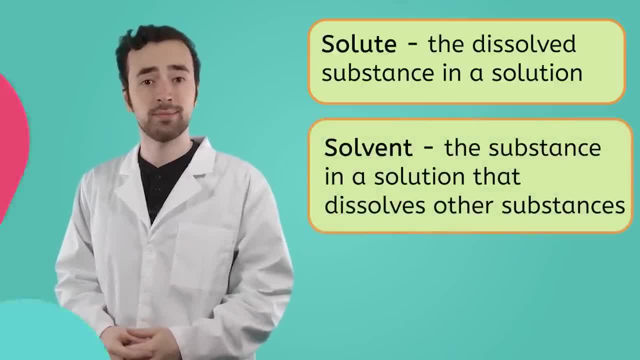 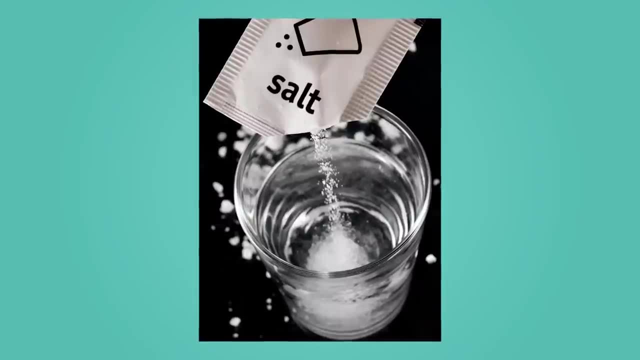 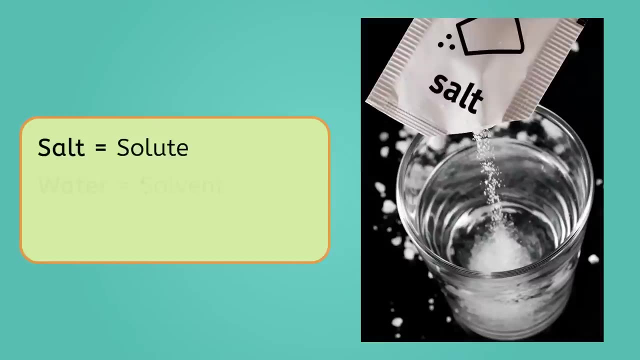 dissolving into is called the solvent. The liquid that dissolves into a liquid is called the solvent. Take salt water, for instance. Salt water is created when salt is dissolved into water. In this case, salt is the solute, or the substance that dissolves. Water is the solvent or the substance that does the dissolving. 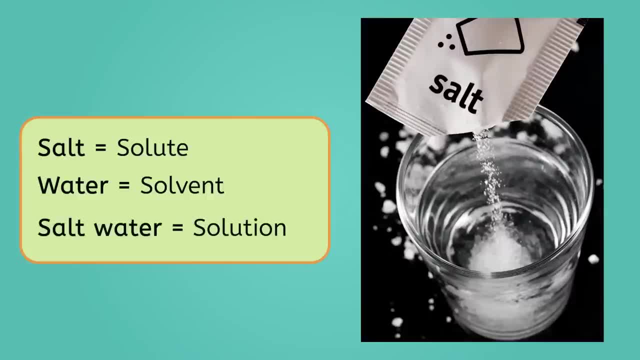 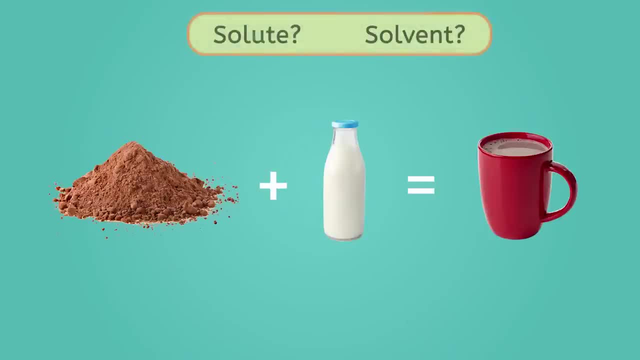 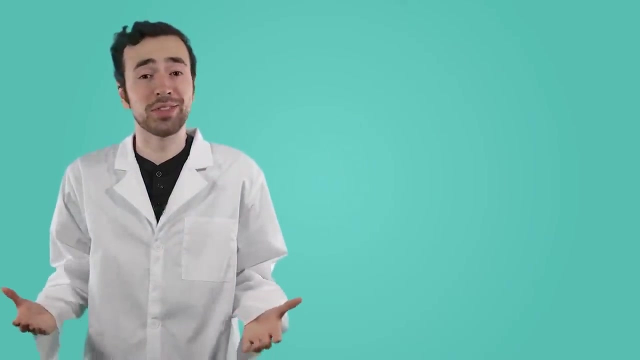 and salt water is the solution. Try one for yourself. If you combine hot cocoa mix with milk, what's the solute And what's the solvent? Pause the video here to write down your answer in your guided notes. Solutions don't even have to be in the liquid state. There are solid solutions. 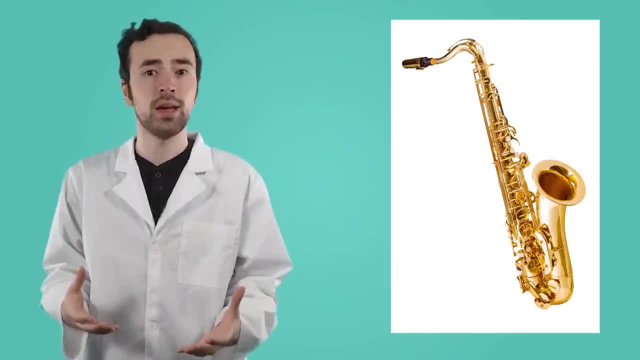 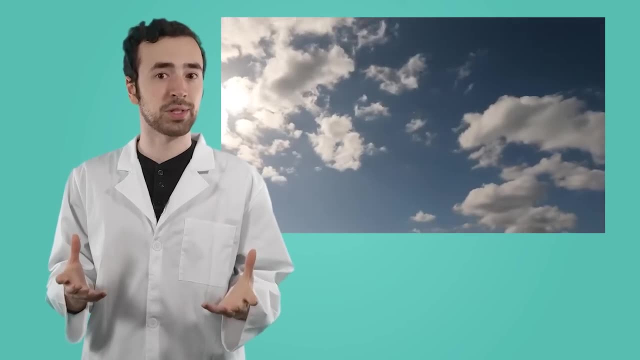 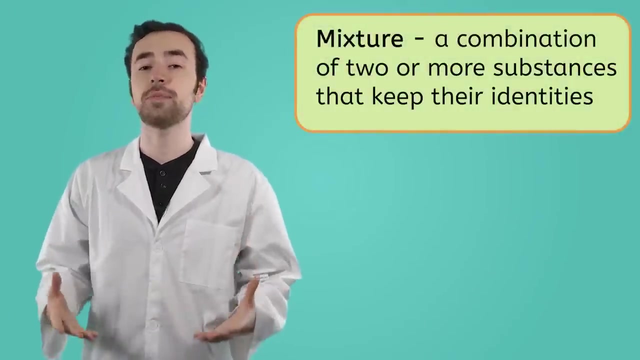 like the copper and zinc solution that makes up brass. And there are gas solutions too, like the mixture of oxygen, nitrogen and carbon dioxide that makes up our atmosphere. So a mixture is a combination of different substances that each keep their identities. 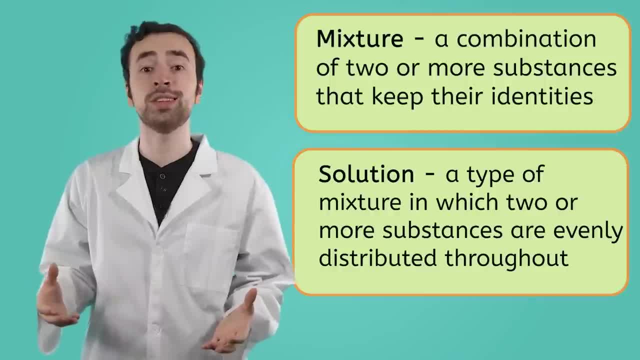 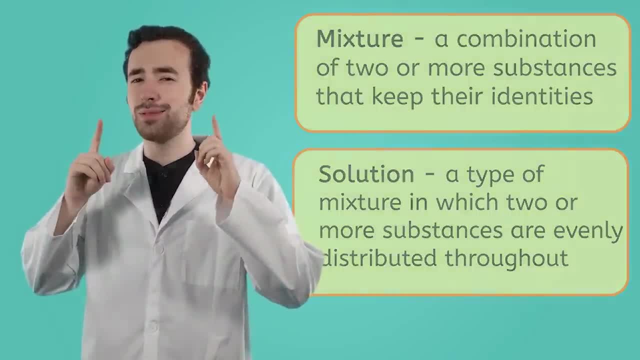 And a solution is a mixture in which the different substances are evenly distributed throughout it. But what happens when we don't want the mixture to be a mixture anymore, Like with that sandy, salty sippy cup full of water that my sister made? 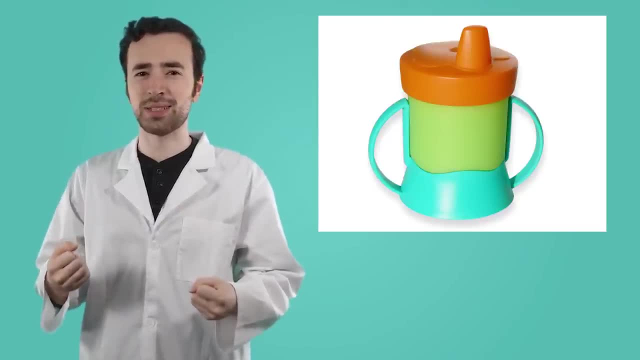 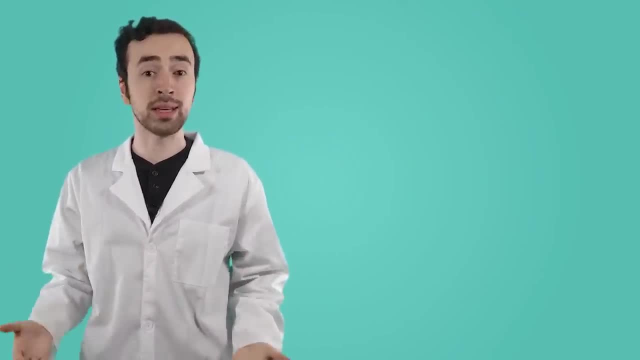 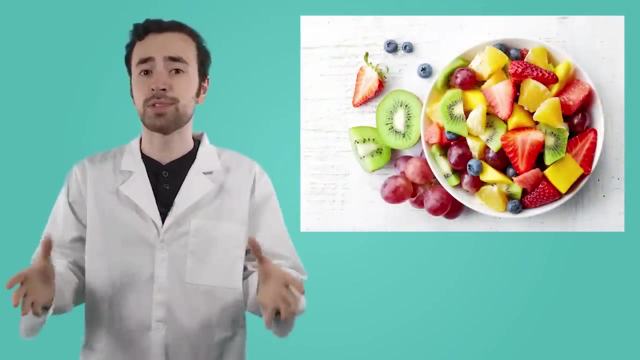 Well, some mixtures can be separated pretty easily, Like, say, a fruit salad. If you wanted to separate that, you could just take your fingers and pluck out all the different kinds of fruit and separate them. that way It'd take forever, but it's easy. However, not all mixtures can. 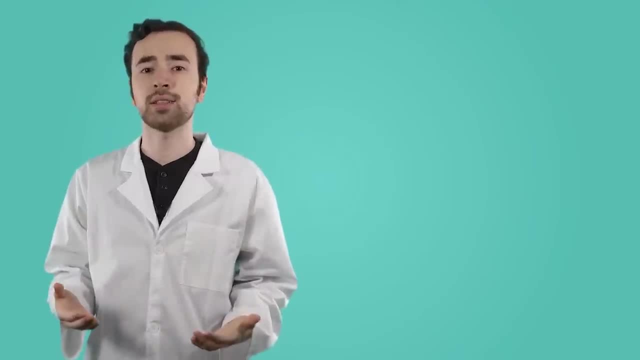 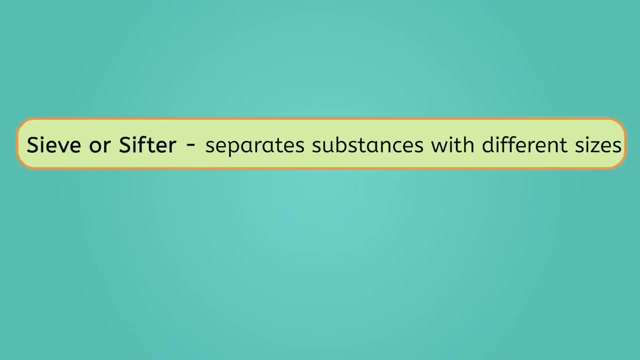 be separated. so, simply, When that's the case, we can use the physical properties of matter to separate them. For instance, if substances in a mixture are different sizes, we can use a sieve or a sifter to separate them, Like with this mixture of sand and gravel. 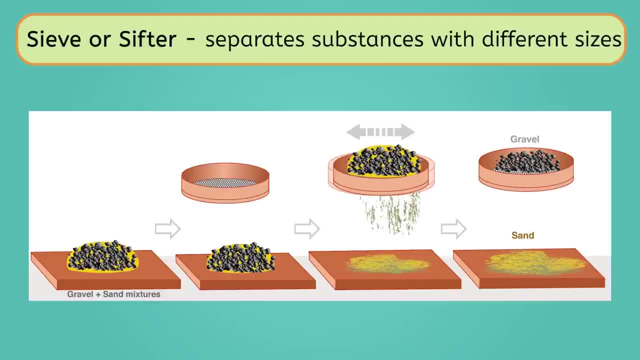 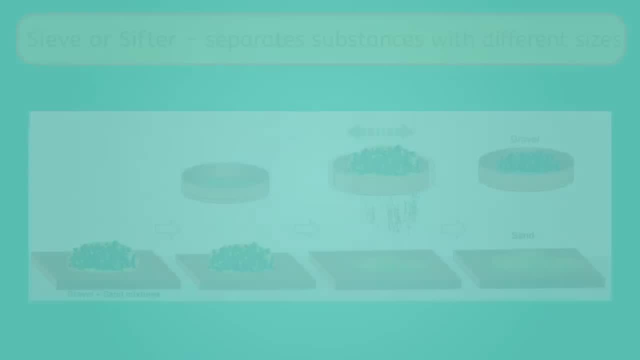 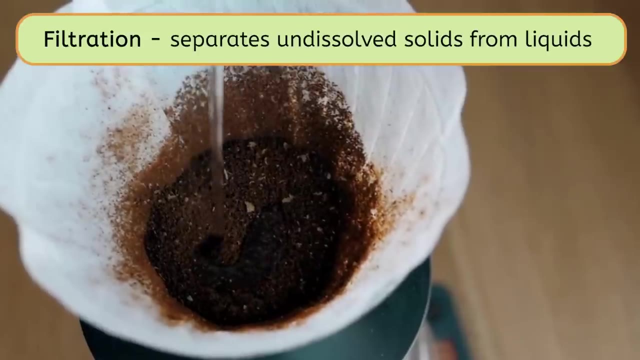 The small pieces of sand will fall through the holes and the larger pieces of gravel don't. Similarly, we can use a process called filtration to separate solids and liquids. The liquids will move through the filter, but the solids cannot. You might see this process being used when you're. 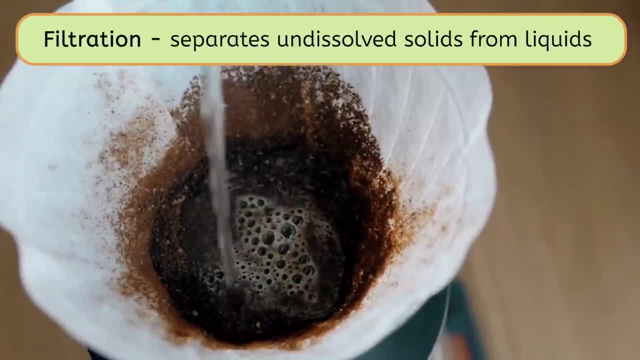 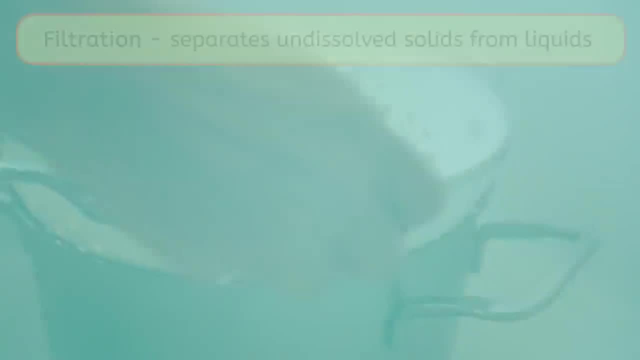 parents filter coffee grounds from their liquid coffee, or when noodles are separated from the water they were cooking in. We can also use physical properties like magnetism to separate mixtures. For example, how do you think we could separate a mixture of sand and iron filings? 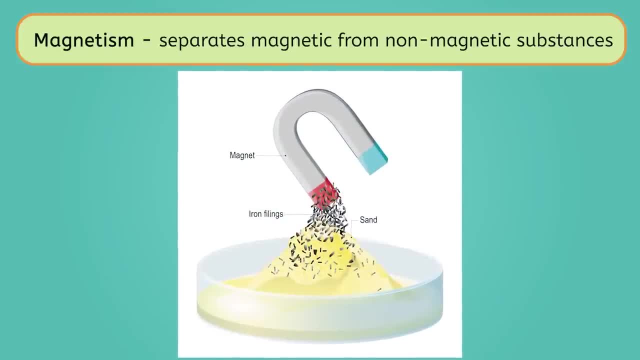 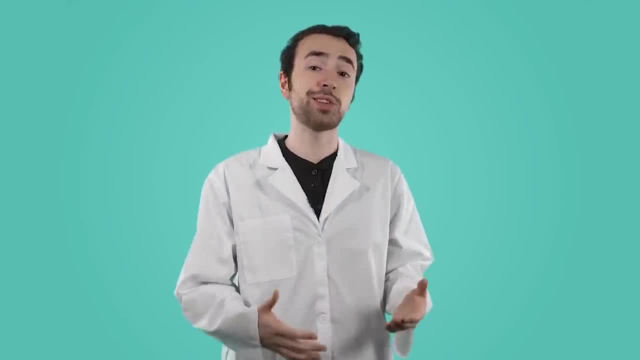 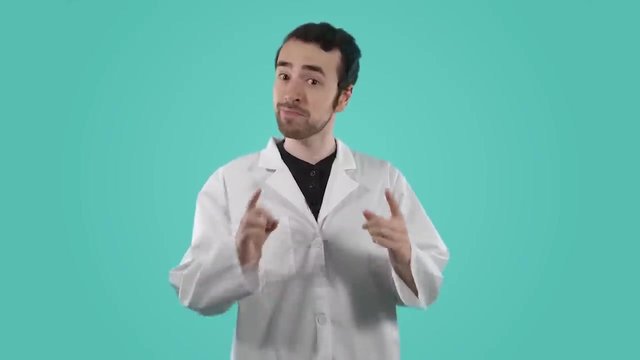 Sure, we could use a magnet to attract all the little bits of iron leaving the sand behind. So far, all of our examples have been mixtures but not solutions. Solutions are usually much more difficult to separate than other kinds of mixtures, but they're not impossible. One. 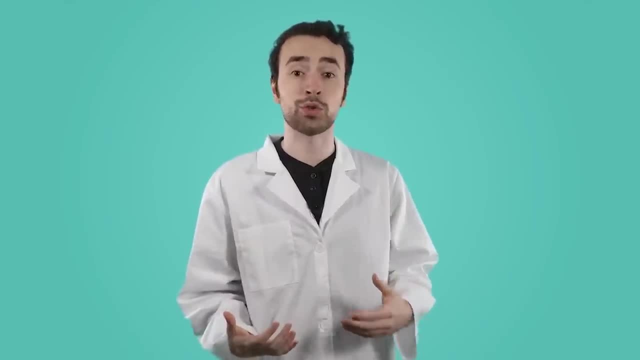 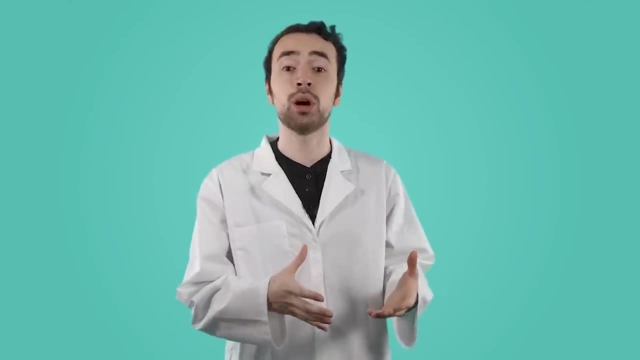 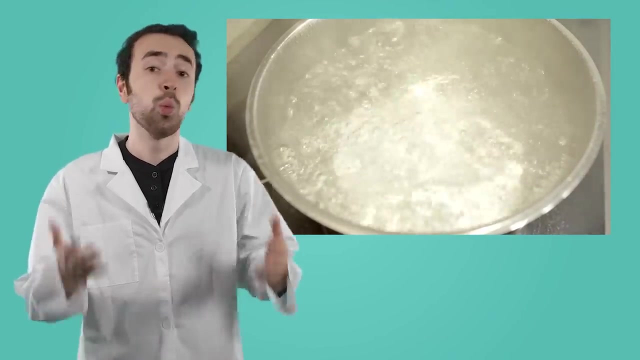 of the most useful physical properties to know when we're trying to separate a solution is the boiling point of each of the substances. For example, let's say we have a solution of water with solid sugar dissolved into it. We could just boil the whole thing on the stove. Water's boiling. 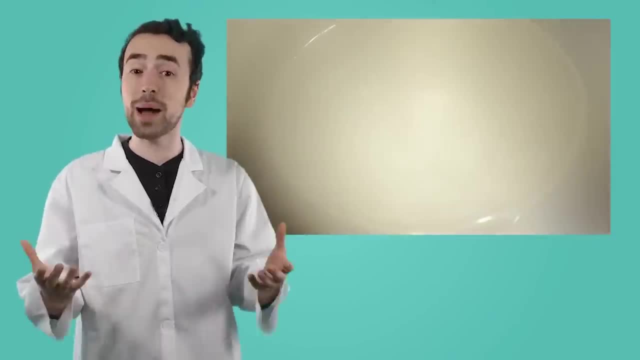 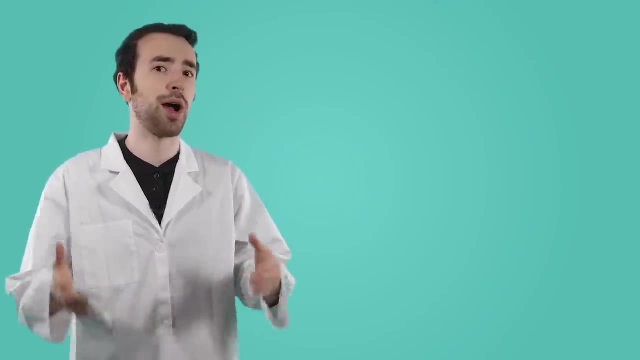 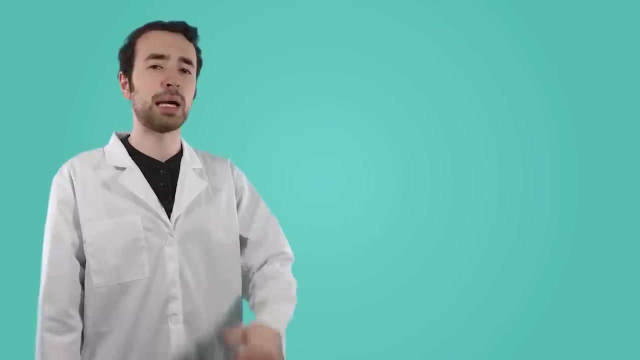 point is much lower than that of sugar, so the water will evaporate, leaving solid sugar behind. Also, you should know that some solutions will require more than one step to completely separate, And I think that's probably what's going to happen with my sister's water mixture.